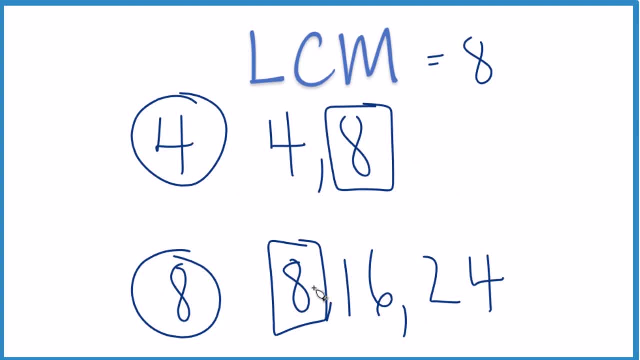 so on, or you can just add them together to get those multiples. That's it. This is Dr B looking for the LCM for 4 and 8.. The answer is 8.. You can do this other ways, but you'll.